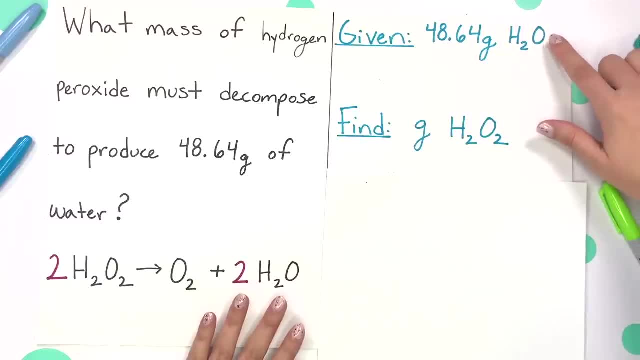 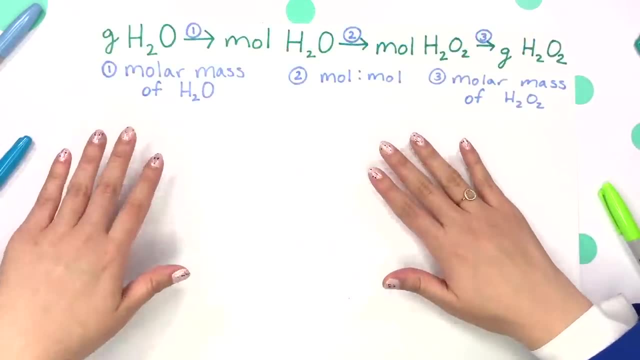 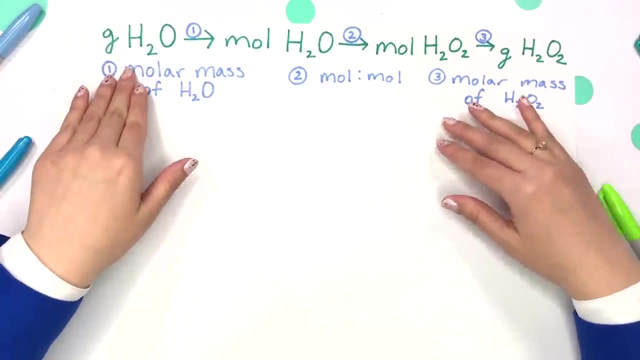 equation, because we're trying to get from grams of H2O to a completely different compound of grams of H2O2.. Our plan is to go from grams of water to a completely different compound of grams of H2O2.. Now we can't just instantly go to grams to grams. We have to go from grams to moles and then moles. 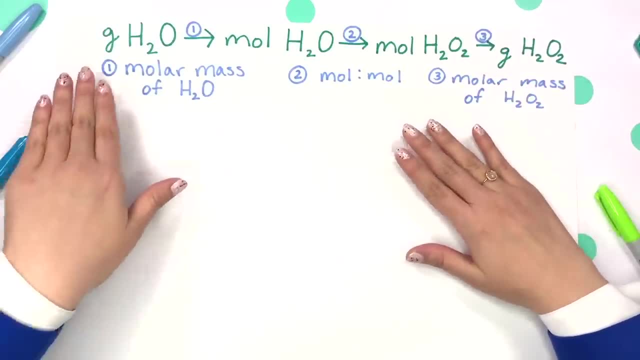 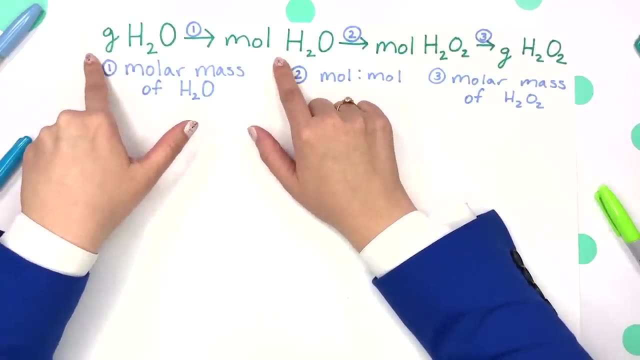 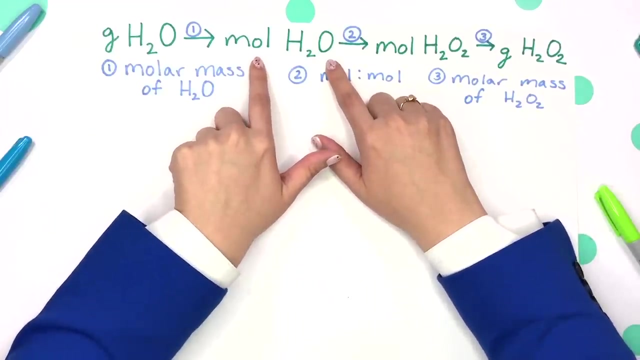 to grams. So our first step is to convert our grams of water to moles of water using our molar mass. Whenever we go from grams to moles, we use the molar mass of that compound. Then, once we have our moles of H2O, we will change our compound entirely, using our molar mass of H2O. So we're 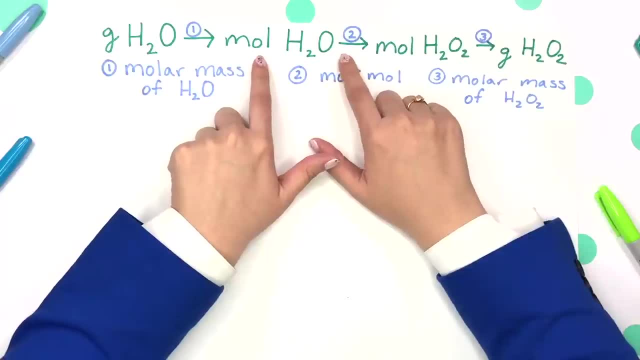 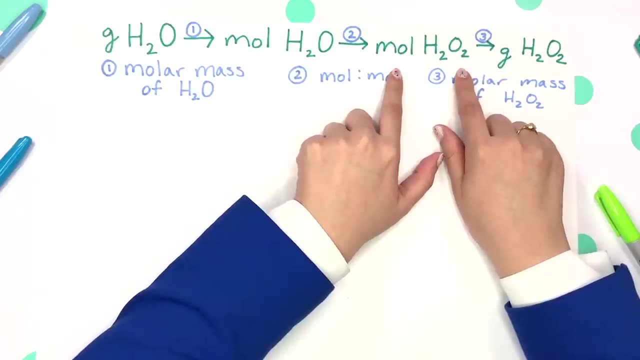 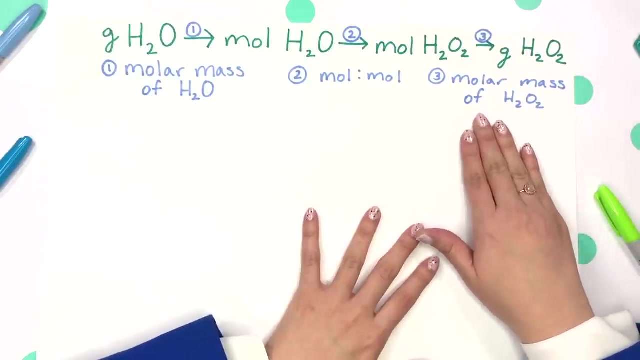 going to go from our moles of water to moles of hydrogen peroxide. Now that we have our moles of hydrogen peroxide, we can then convert that down to our grams of hydrogen peroxide, once again using our molar mass of that compound. So let's set this up. You want to put your given on top? 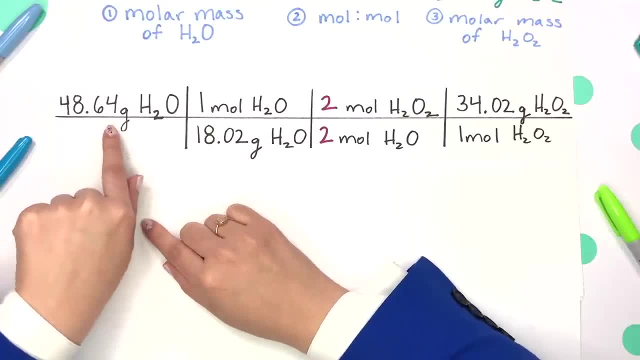 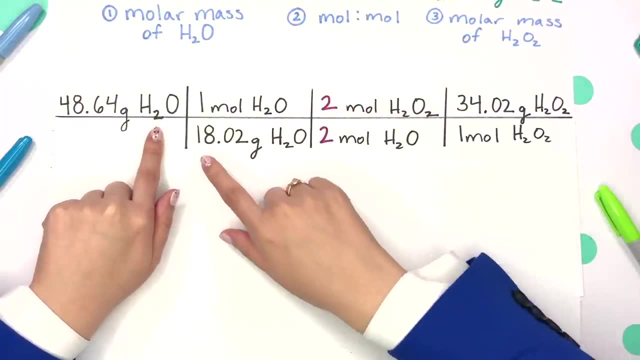 That's what you always start with, is your given. So we have our 48.64 grams of water and we're going to use that first conversion factor as our molar mass of water, and it's going to be 18.02. 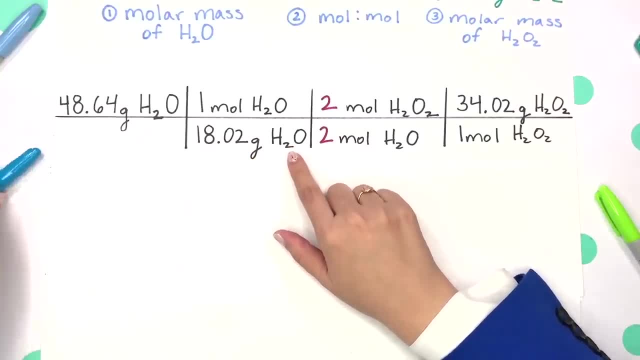 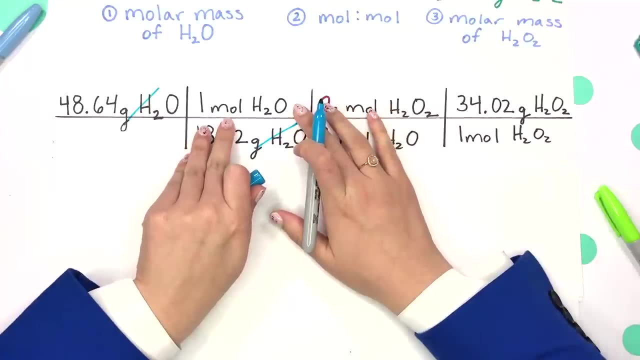 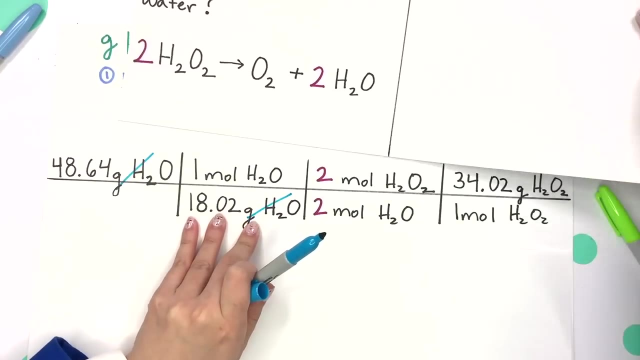 grams. You align these two across from each other, because then we will then cancel out our grams of water. We now are left with moles of water and we're going to go back to our balanced equation to do a mole to mole ratio. So, looking back at our balanced equation, we see that we have two moles. 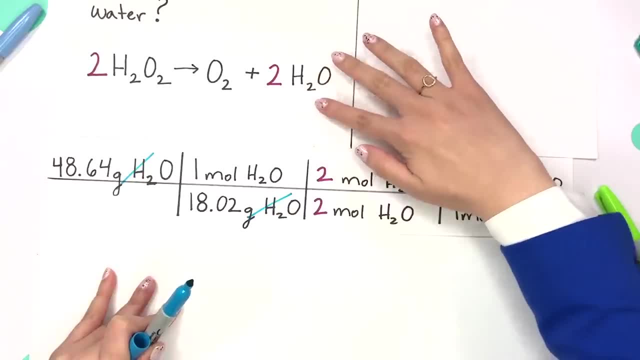 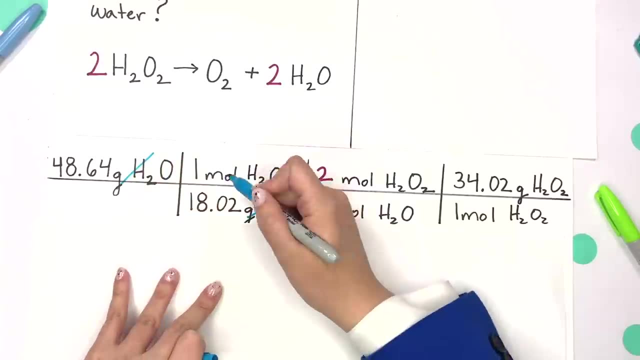 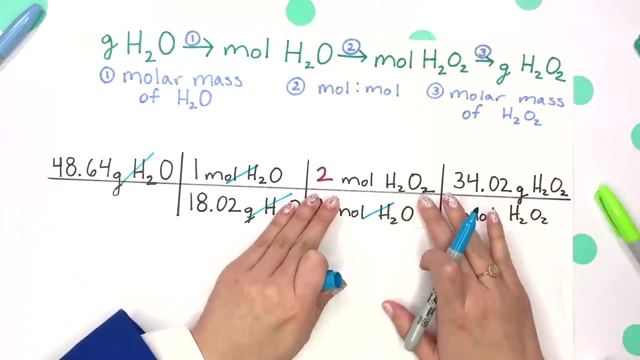 of hydrogen peroxide and per every two moles of water. That's also why I put the two moles on the bottom, so they can then cancel. Those moles of water would then cancel and we're at moles of hydrogen peroxide Now from moles of hydrogen peroxide. we will then use our last conversion. 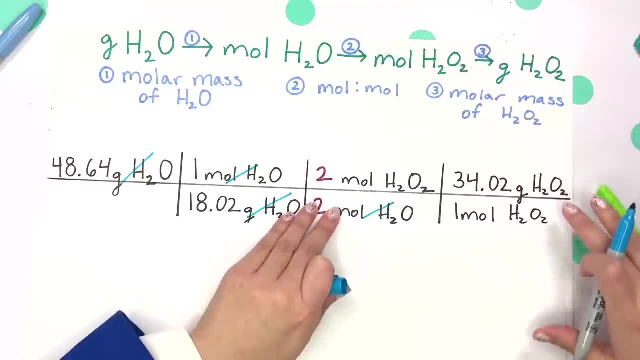 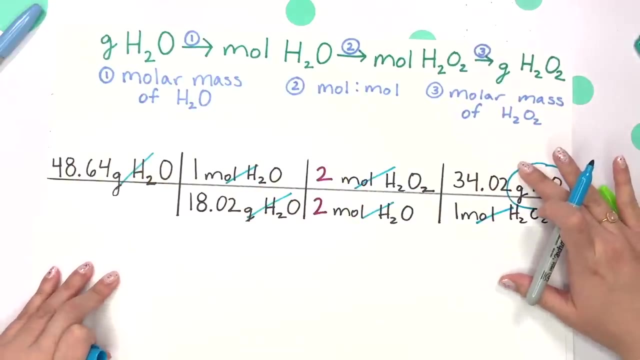 factor the molar mass of hydrogen peroxide, to get to grams of hydrogen peroxide, because our molar mass would be left with just the grams of hydrogen peroxide, which is what we're solving for. So multiply straight across, divide by that, 18.02 times the two, and you get. 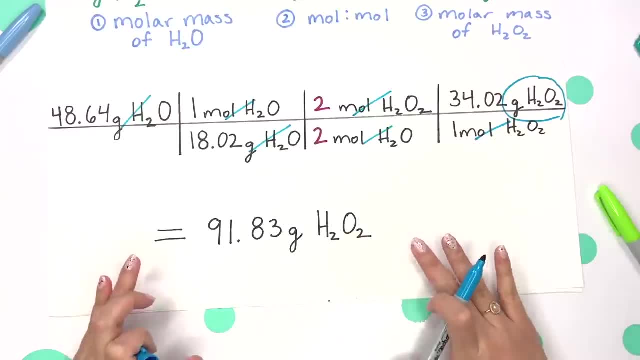 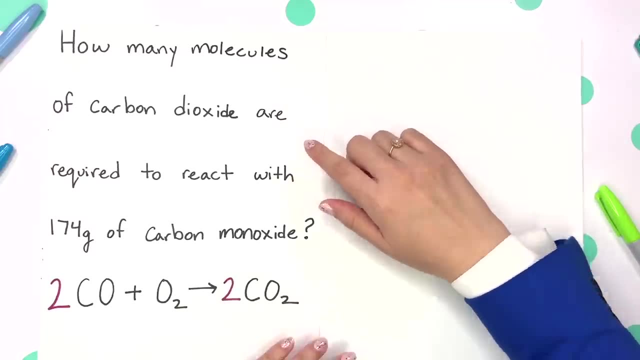 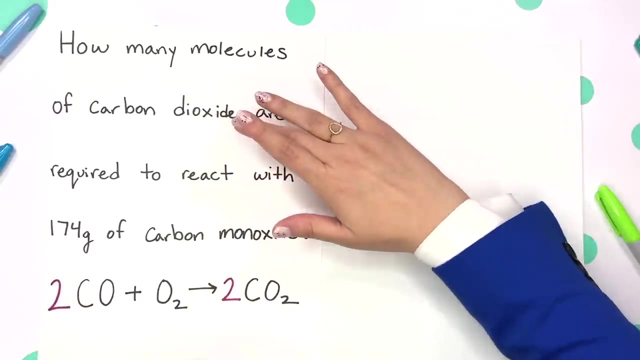 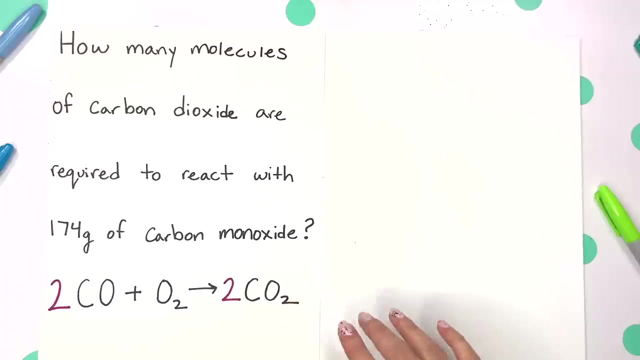 91.83 grams of hydrogen peroxide. Our next example states how many molecules of carbon dioxide are required to react with 174 grams of carbon monoxide. So remember that carbon dioxide, that di, meaning two, is our CO2.. Carbon monoxide, mono, meaning one, is our CO. So let's 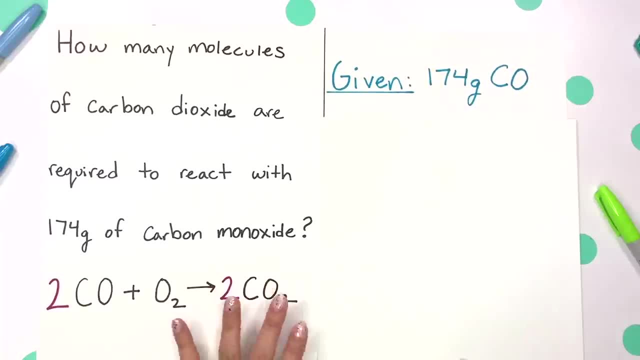 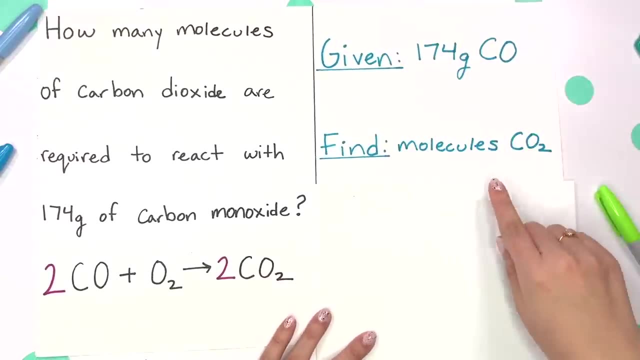 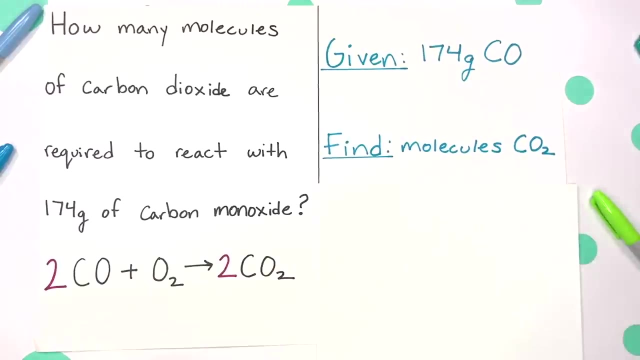 identify what we're given and what we're solving for. So we're given the 174 grams of carbon monoxide or CO, and we are finding molecules of CO2.. Key word right there: molecules. So remember anytime you see that word molecules, you use Avogadro. 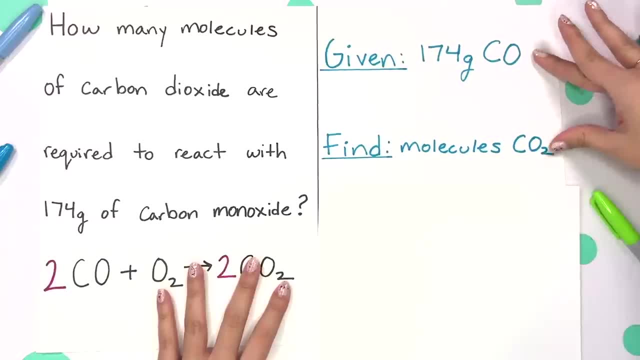 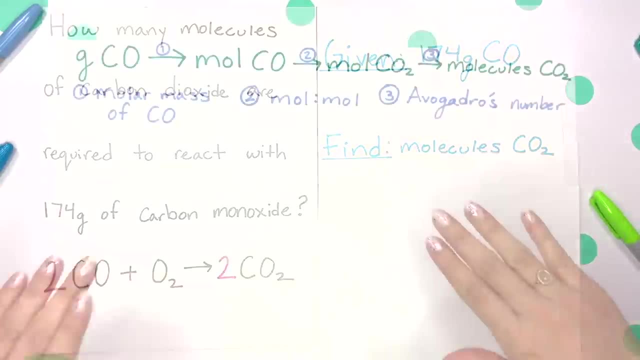 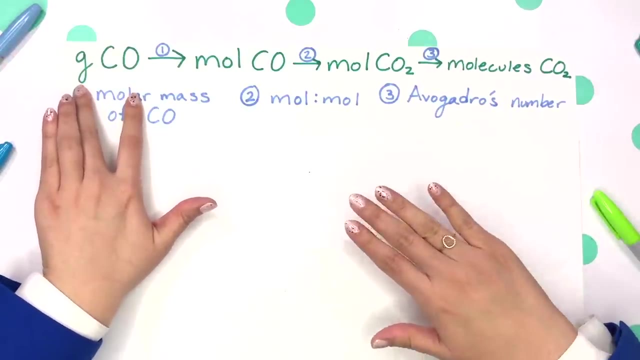 Number. Also, we're changing our compound, So we have to use a mole to mole ratio. using this balanced equation, Let's set it up. Setting up our plan, we see that we're going from grams of CO or carbon monoxide and we're trying to get to molecules of carbon dioxide. So we're changing. 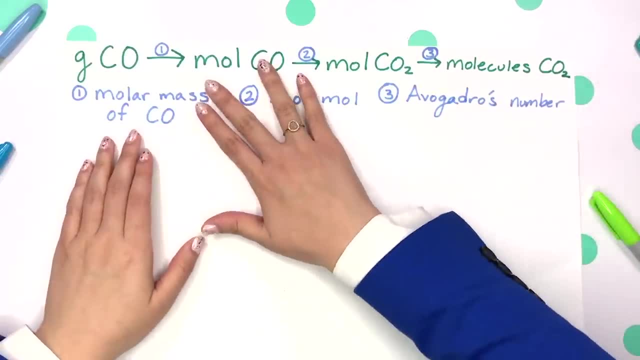 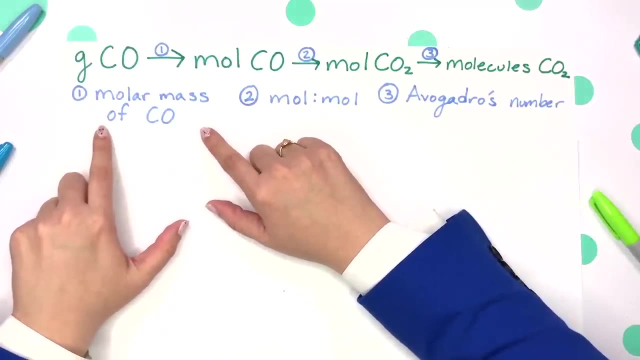 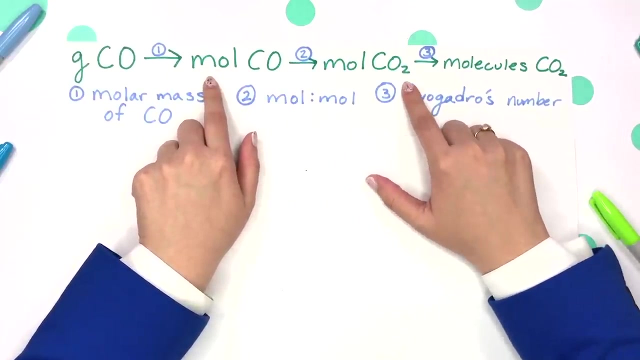 our compound, We have to convert first to moles of carbon monoxide. So from going from grams to moles, we use the molar mass of carbon monoxide. That's our first conversion factor. Then, now that we're at moles of carbon monoxide, we will change our compound to the moles of carbon dioxide, using 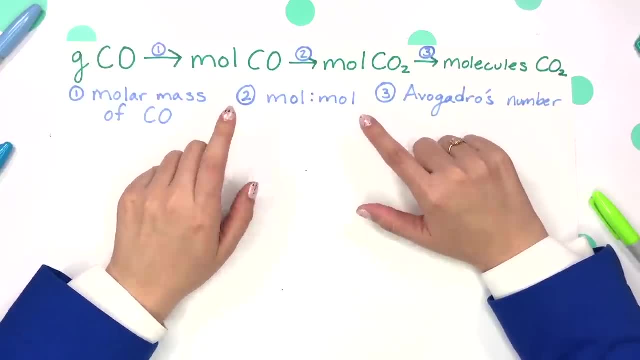 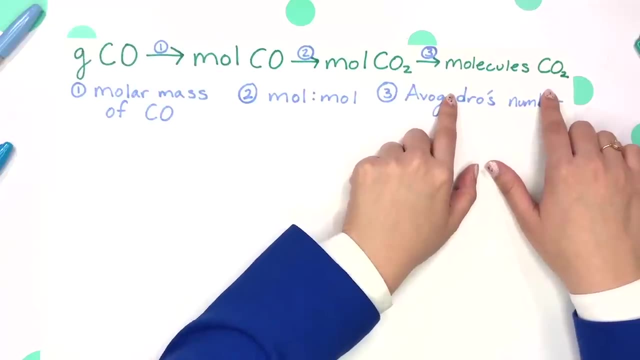 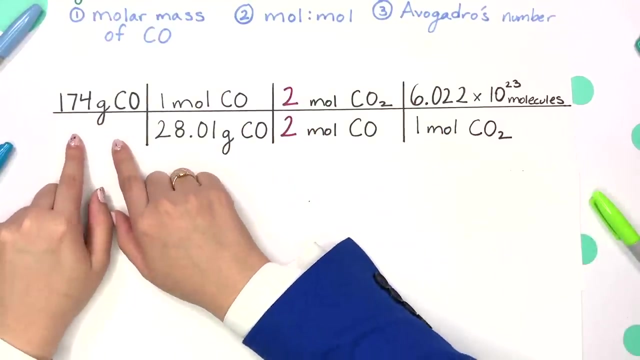 our balanced equation, using that mole to mole ratio. Now that we're at moles of carbon dioxide, we can then convert this to molecules of carbon dioxide using Avogadro's number. Your proper setup would then begin with our grams of carbon monoxide. 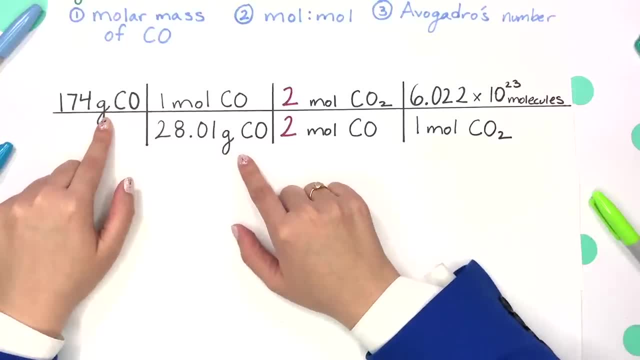 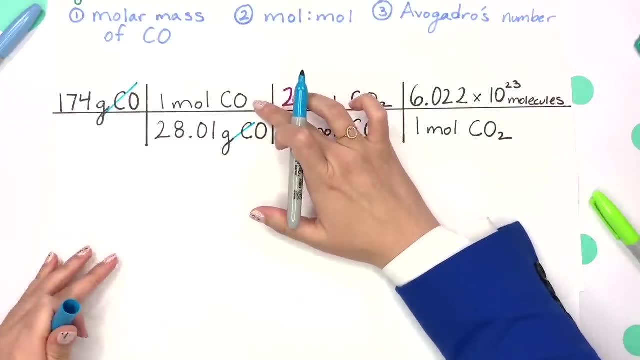 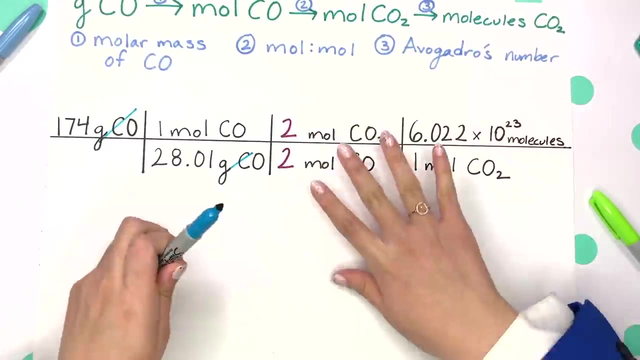 because that was our given, and then aligning those grams across from each other so they can then cancel. We would then get moles of our carbon monoxide. Next we're right here on our second conversion factor, where we have to use our balanced equation. So these numbers, if we go, 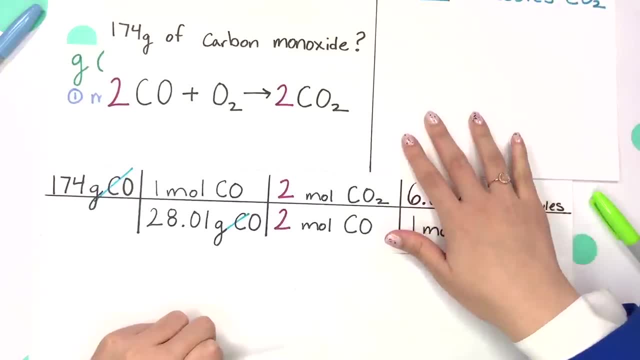 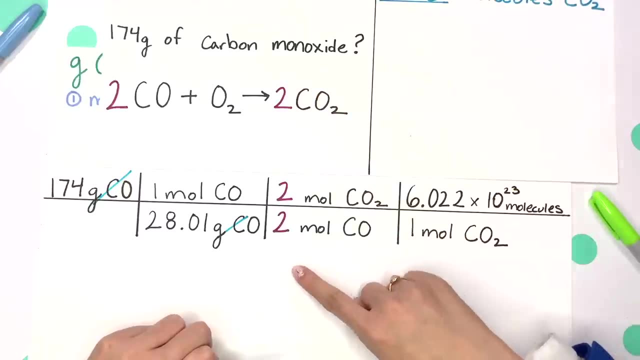 back to our balanced equation. we would then see that that two moles of carbon dioxide came right here from the coefficient from our balanced equation. This other two came from right here, the other two on our balanced equation. That's where we get our moles to mole ratio from Align those moles across from each other, specifically the moles.